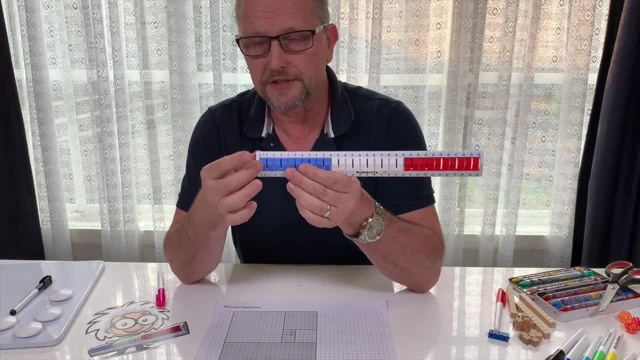 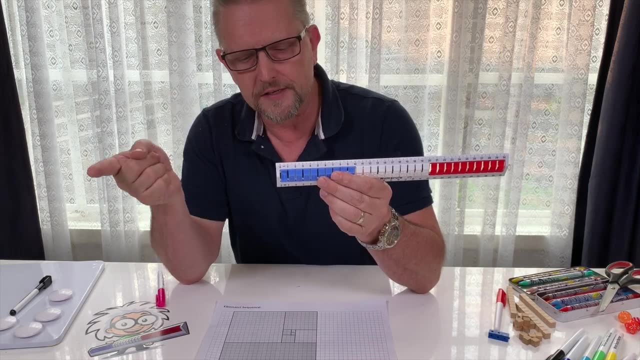 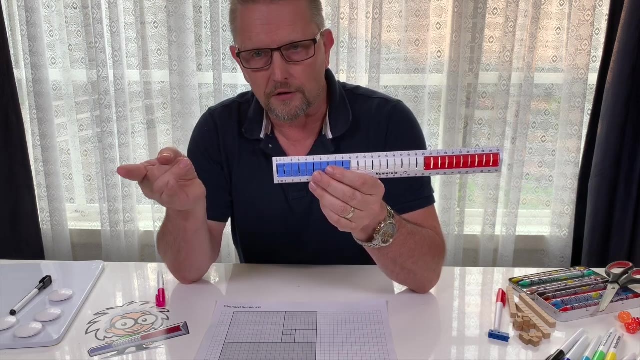 and what we do is we start the sequence off by adding on one, okay, and then what you need to do is add on the previous number to the one that you actually have there. all right, So we have zero, we add on one and we get one. all right, I'm going to write this Fibonacci sequence here. 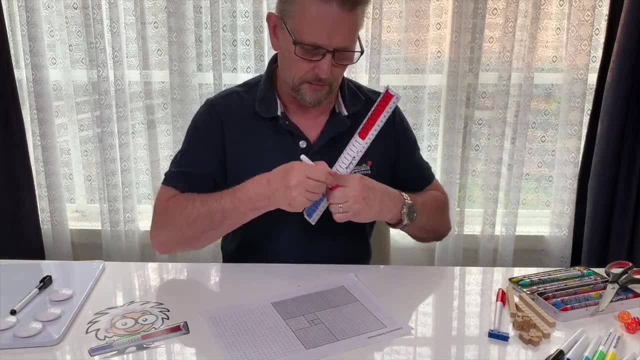 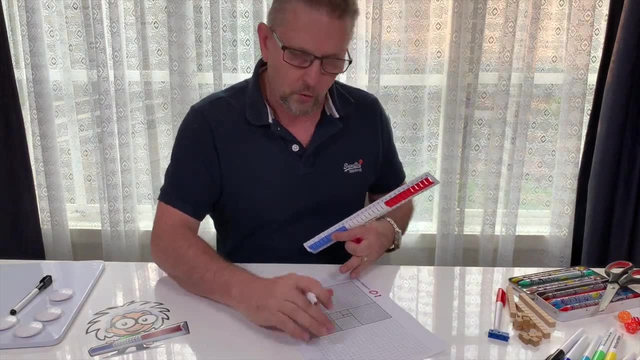 because we're going to do it in a different way. So we're going to do it in a different way and we will use it later. I'll turn this back around in a minute. So we started with zero, okay, then we added on one. Now we add on the previous number. In this case, 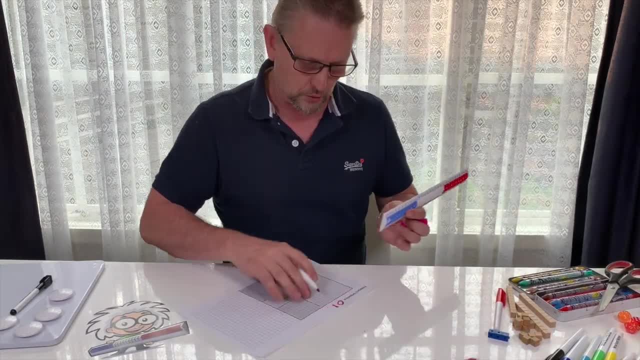 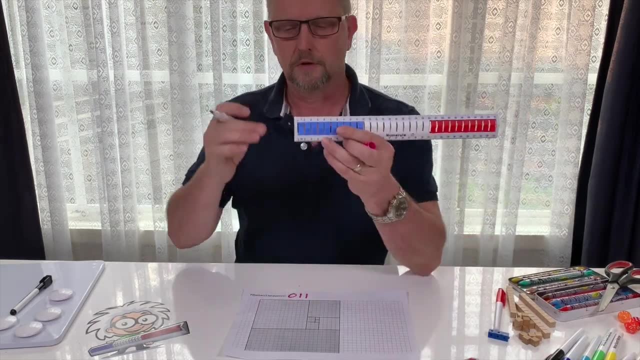 the previous number is zero. So zero plus one is one. So in the Fibonacci sequence we have zero and then we have two ones. all right, So we're still at one. In the next part of the sequence we add on the previous number. So we're still at one. So we're still at one. 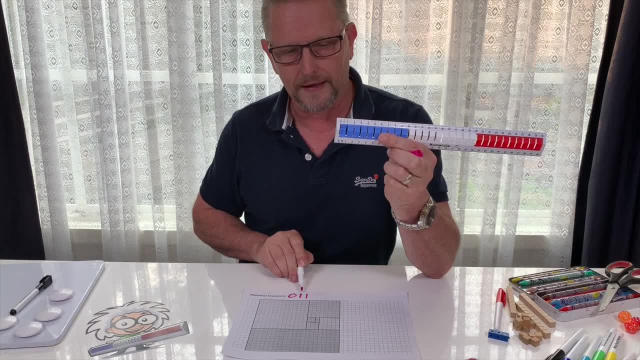 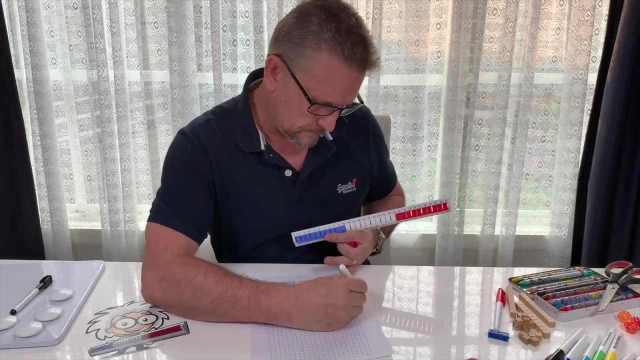 So we're at one and we're going to add on one again. So one add on one is two. So let's write that one down Two, All right. So now we're at two. we need to add on the previous. 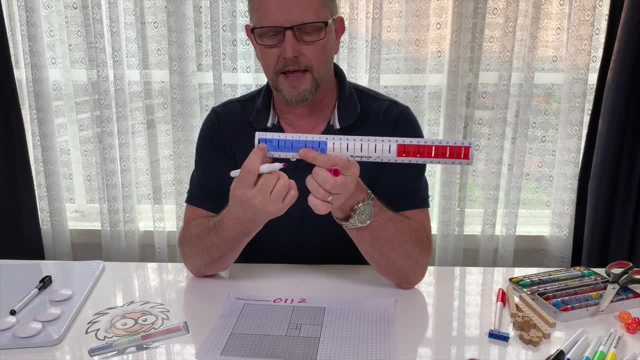 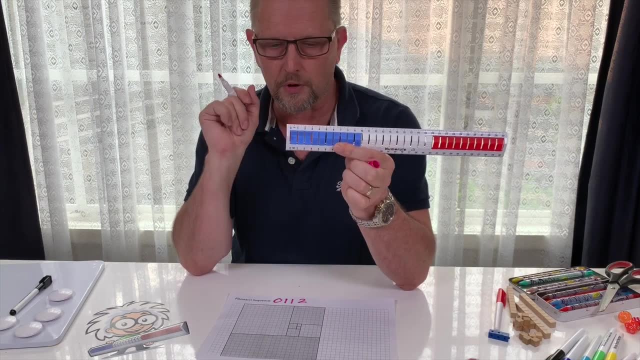 number. Well, on the ruler here you can see what the previous number is right next to the number that you've just pressed down. So it's two add on one and we'll end up with three. Just bear with me for a minute. It'll make sense in just a second, All right? 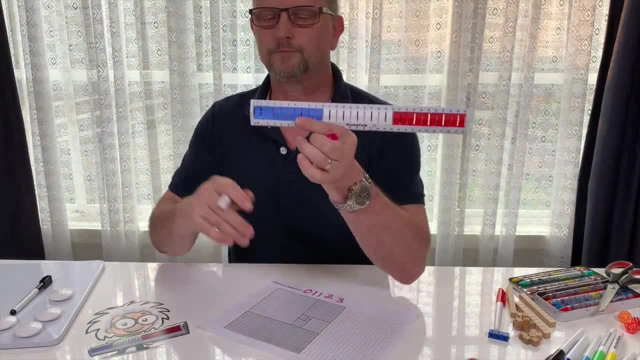 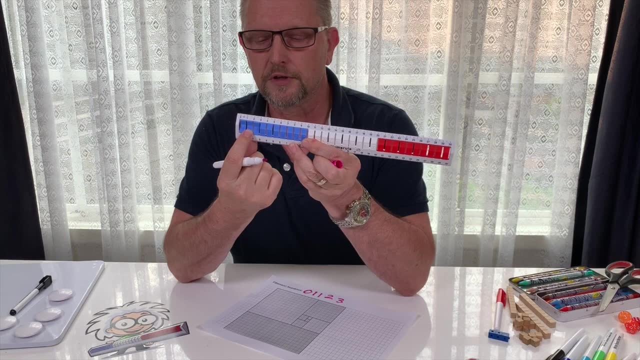 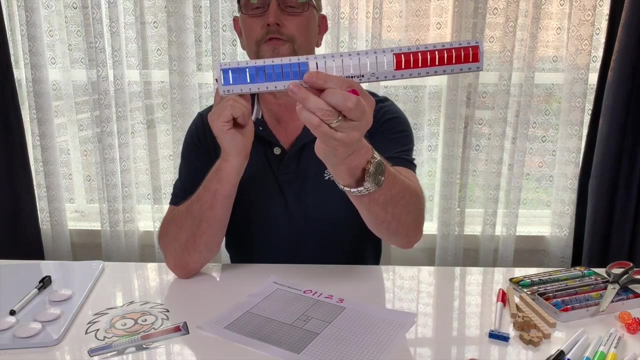 So let's write that down. We're up to three here. So in the Fibonacci sequence, we've got this number and we add on the previous number, which is two, So we've got three. we're going to count on two. Okay, One, two and we end up with five. Can you see that? Let's write that one down: Five. 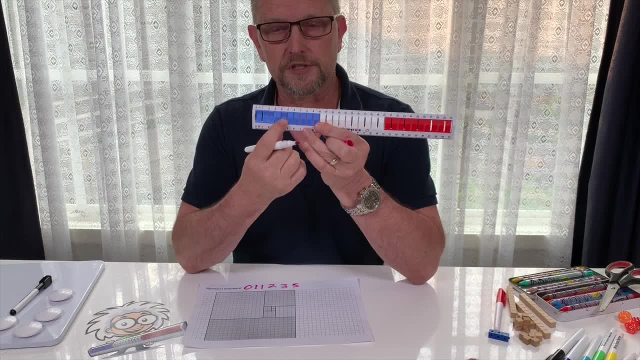 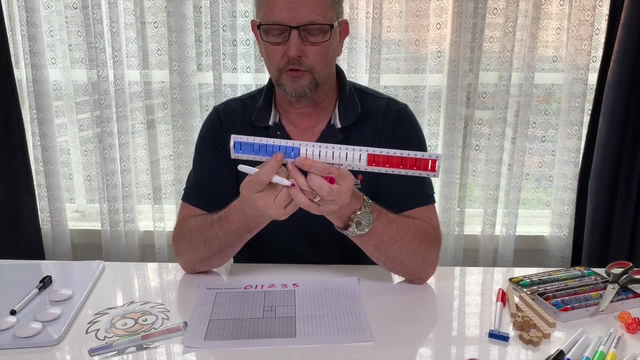 Excellent, All right. So in the Fibonacci sequence we take that number, we add on the previous number, which is three. So five count on three, One, two, three and we end up with eight. Let's write that one down: Eight. 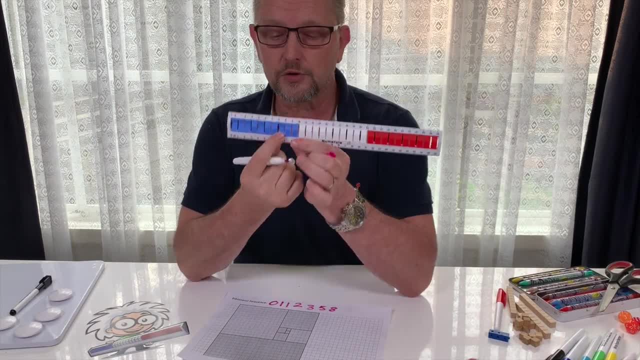 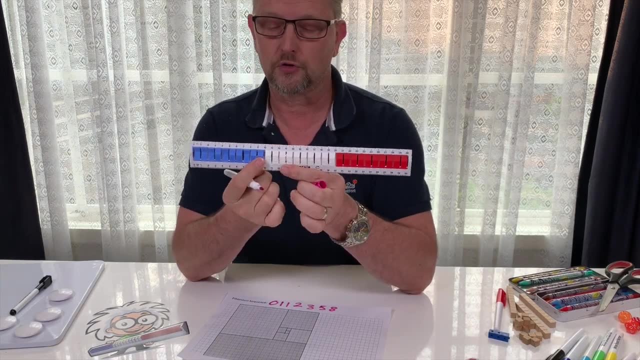 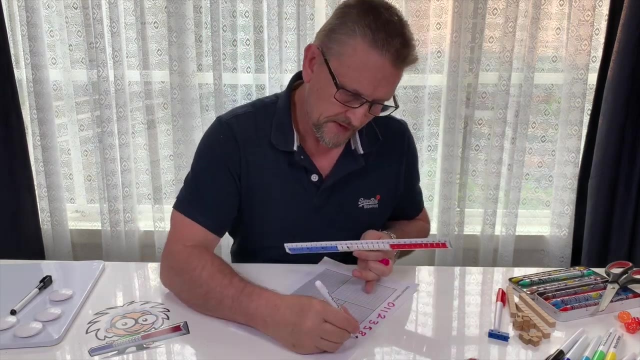 Excellent, All right. So in the Fibonacci sequence we take that number and we add on the previous one. So let's count on five, One, two, three, four, five and we end up with 13.. That's the next. 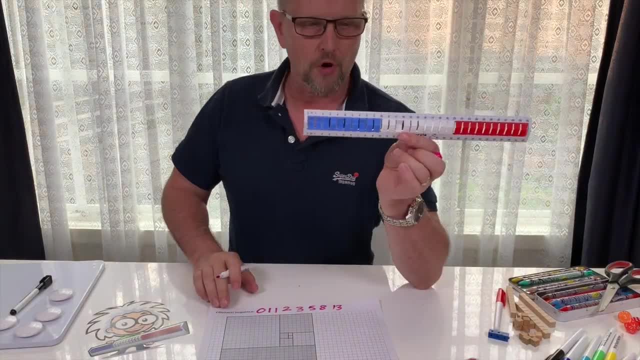 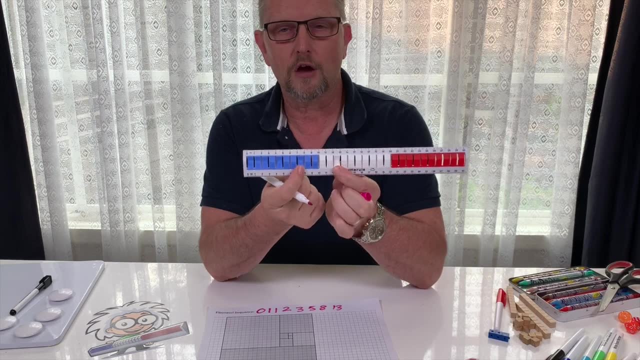 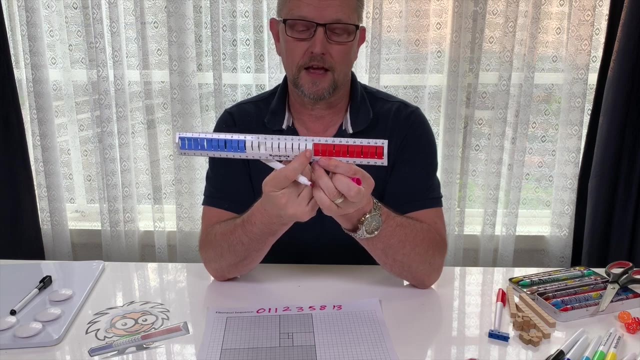 number in the The Fibonacci sequence. All right, So we're at 13.. So we look at the previous number, which is eight. All right, So we're going to count on eight, One, two, three, four, five, six, seven, eight. 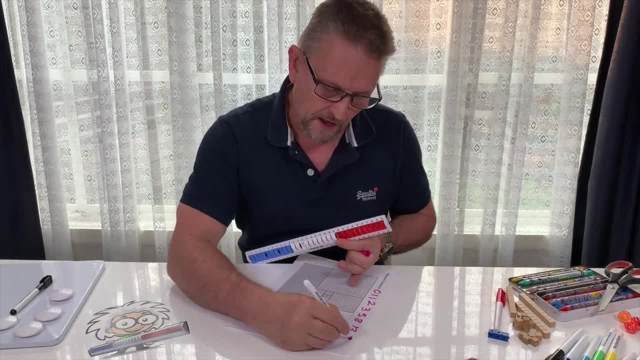 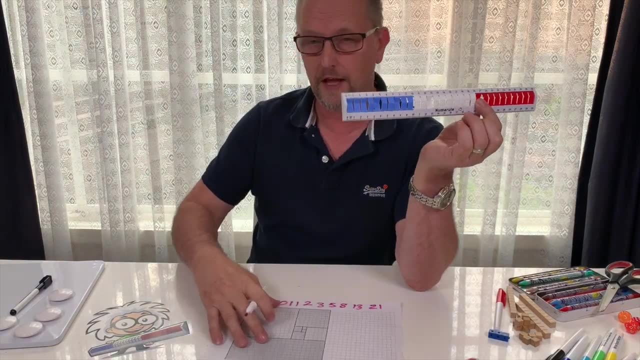 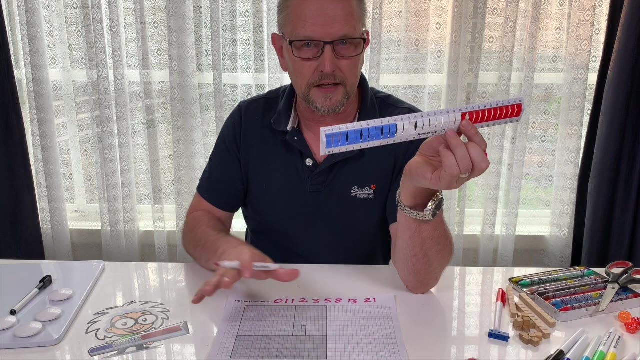 which is 21.. Now, that's about as far as we can go with our numeral as far as the Fibonacci sequence is concerned. But I'll tell you what that really helps to embed that as a concept. And then, when you take this sheet and then you explain an activity further and say: 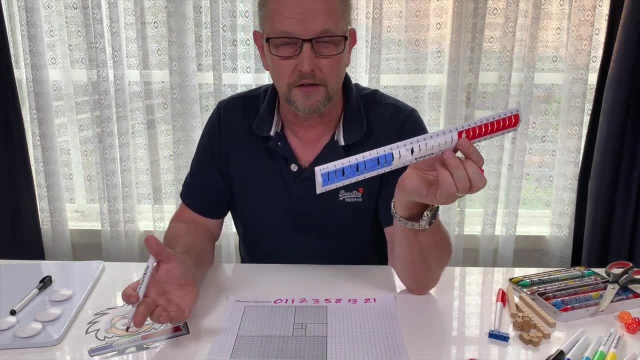 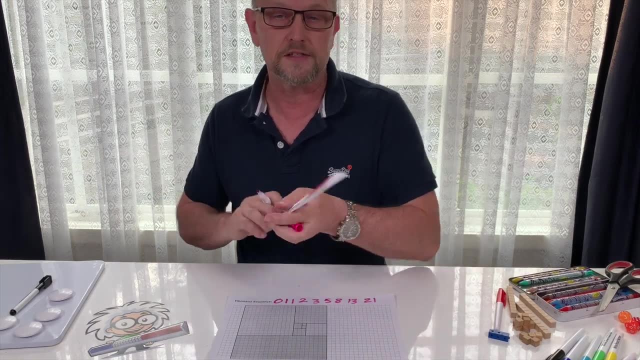 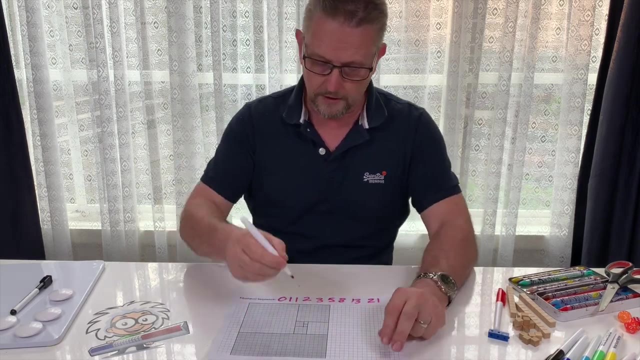 well, we can actually see this sequence out in nature and in various things that human beings make, And let's see what that is. The kids will be actually amazed. So let's have a look at that. So, in the middle of this sheet that I've prepared, we're going to call this our zero starting point. 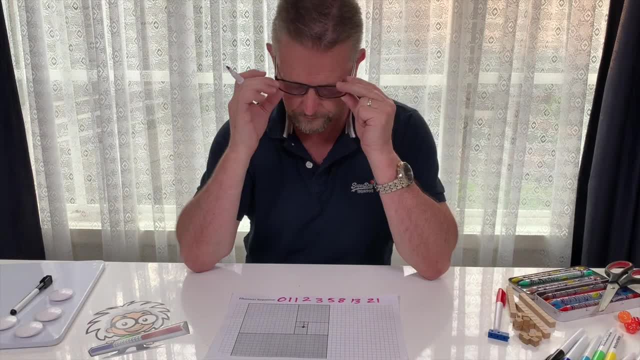 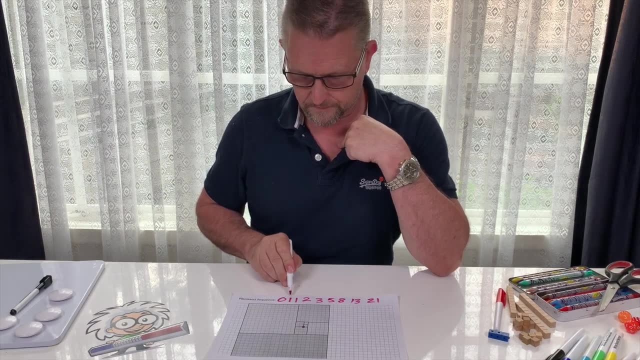 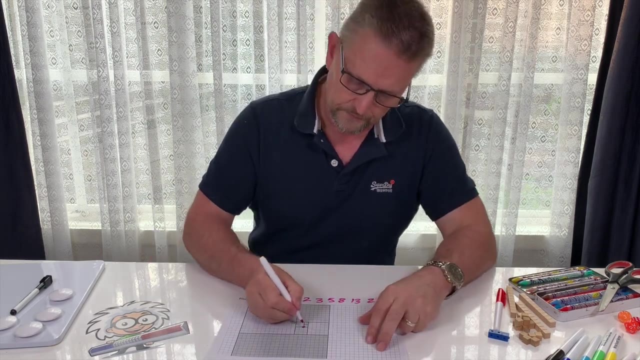 All right, So let's follow our sequence, the Fibonacci sequence. I'm going to use square numbers in this case, So our first one is one. So what we do in this instance is we're going to curve around from one corner to the opposite corner. All right, So this is one times one. You can see that square. 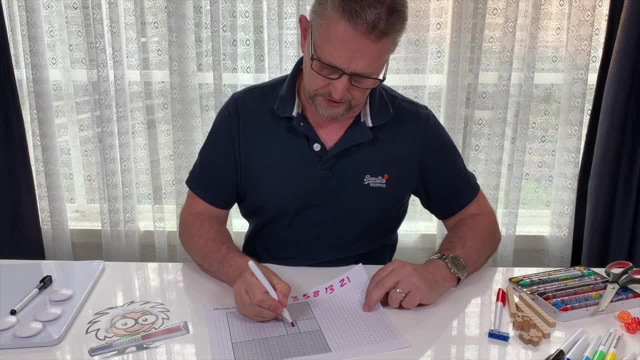 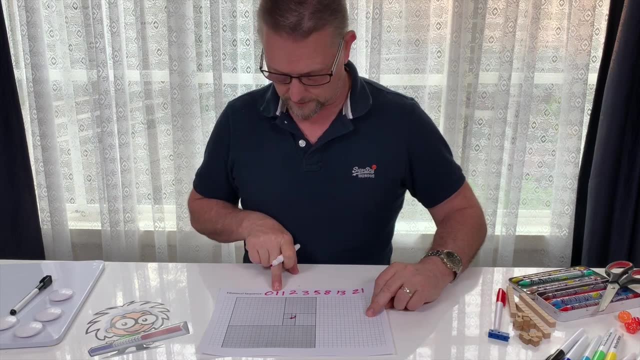 there- Let me hold it up for you so you can see it- And we're going from this corner all the way over to that corner there. Okay, Let's go to our next One, Zero plus one, which is one again. So from here we go, from that corner one times one. 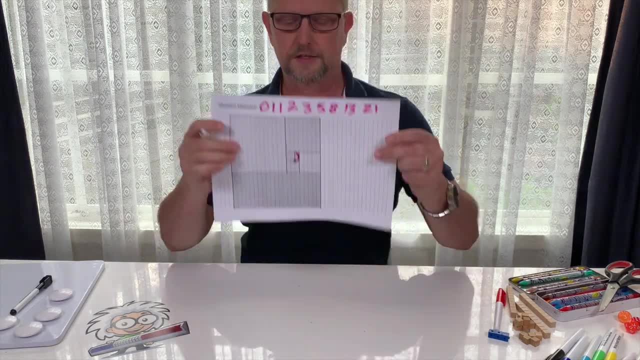 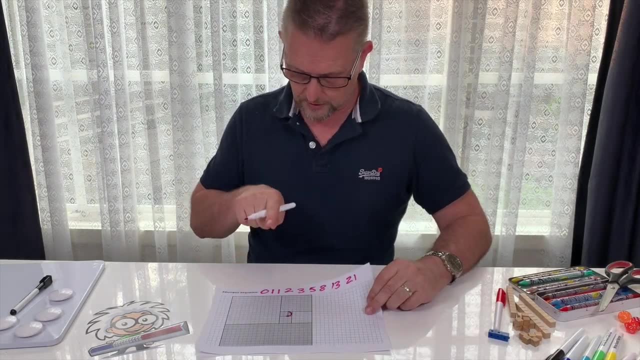 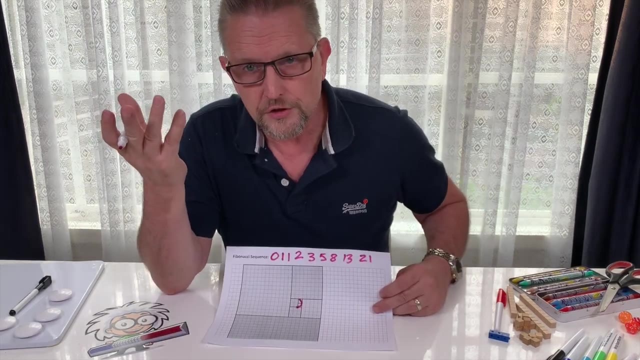 which is one. So one squared, And we go from that corner to that corner there Start making sense. in a minute We'll see what's going to happen. Fibonacci sequence. So we're at one. We add on the previous number, which is one, and we end up with two, Two squared being four. Okay, You can. 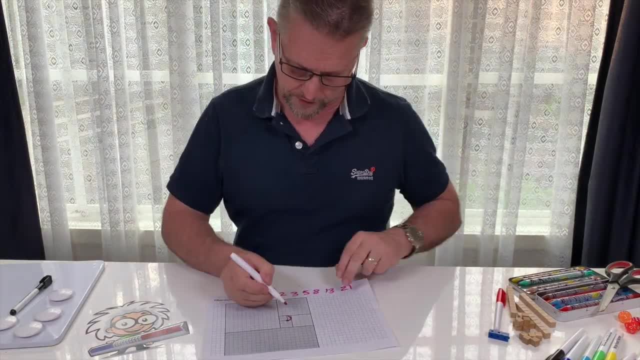 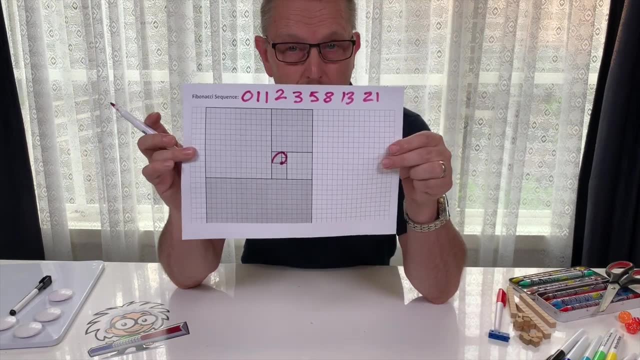 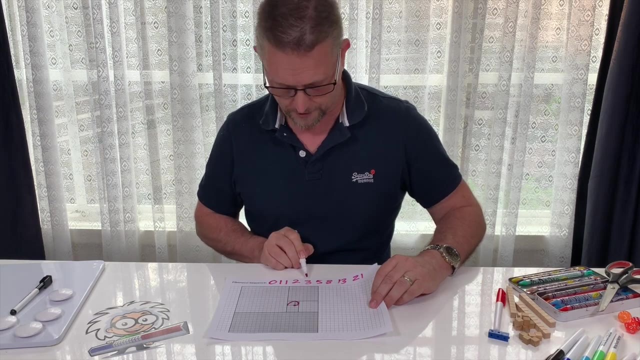 see that square here. So we're at one. We add on the previous number, which is one, and we end up with two. We're going from this corner to this corner. We're following the curve around from corner to corner And see what's happening. Amazing. We're at two. Add on the previous number, Go to three, We end up. 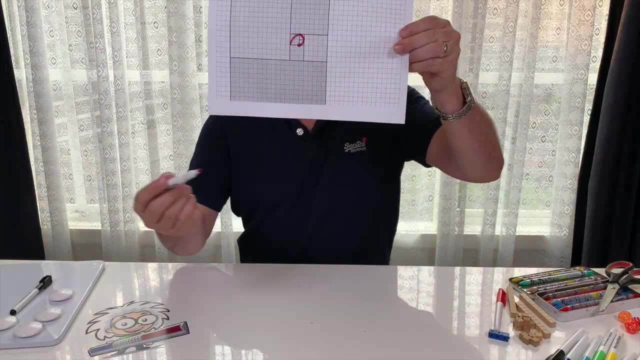 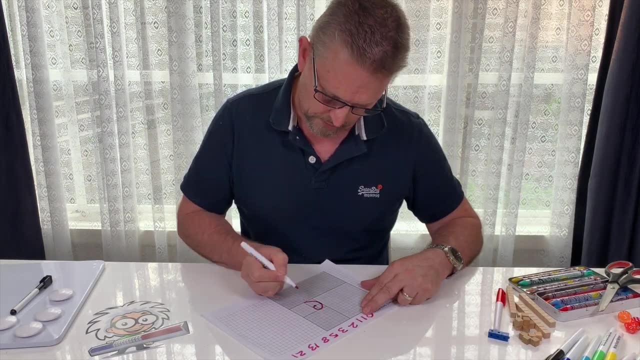 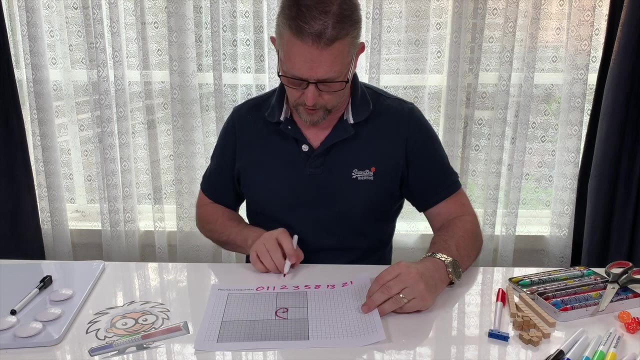 with three, Three times three being nine. You can see the square here And we're going to curve around from that corner, following the same curvature around to the next corner. You can see that the square is starting to take place And then, quickly, we move on to five, because we've 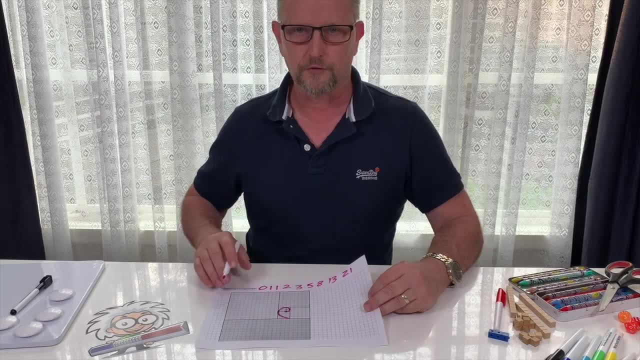 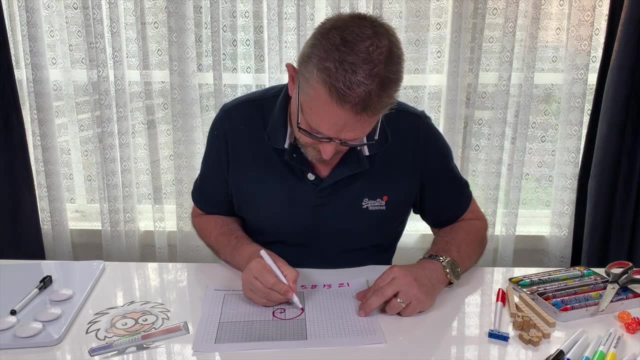 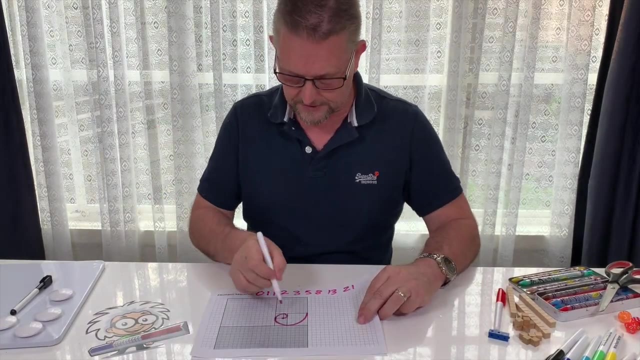 got. we're at three. We add on the two, We get five, Five times five being 25.. And we're going from this corner to this corner, following our curve around like that, One corner to the next, And then we move on to eight, which is obviously 64, which is here Eight times eight, And we move. from this corner, this part of the square, all the way to the next, And then we move on to eight, which is obviously 64, which is here Eight times eight, And we move from this corner, this part of the square, always. 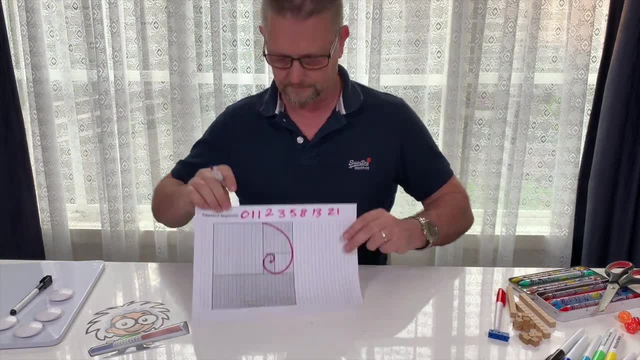 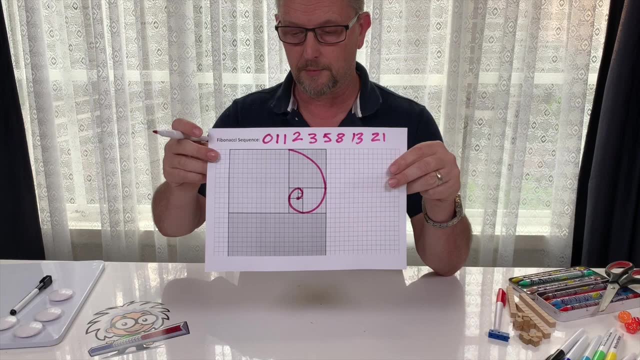 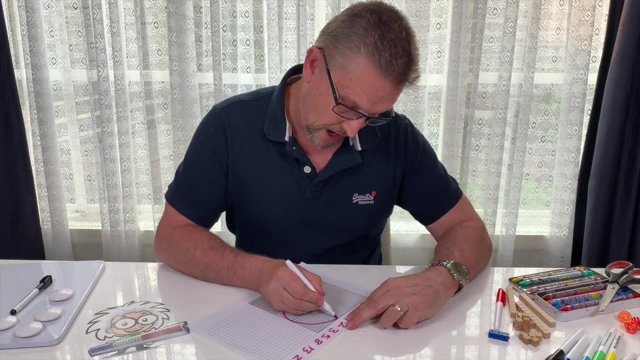 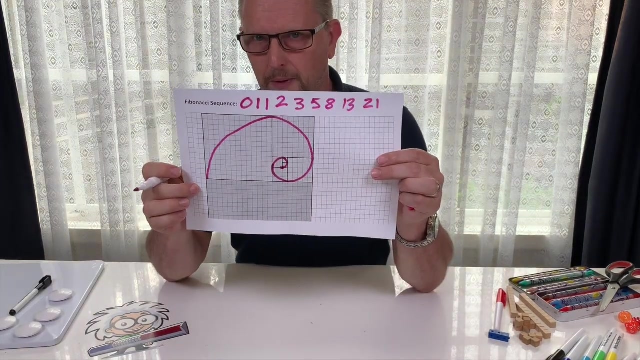 around to the next corner, And then five plus eight, which is 13,. the next one in our Fibonacci sequence, which is 169,, by the way, Move all the way around following the curve from this corner to this corner. I'm going to turn this around so I don't make a hash of it. Could be a bit more. 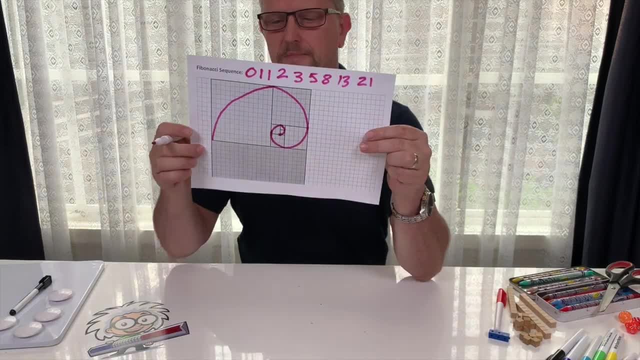 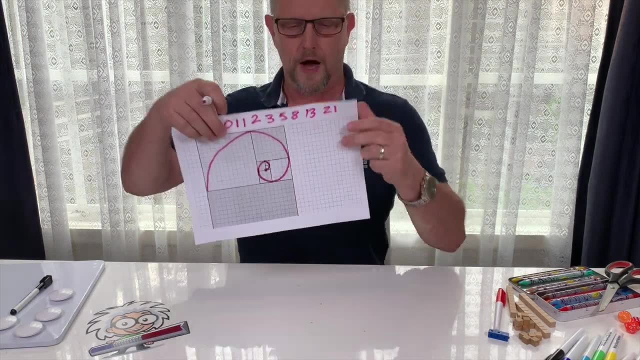 curvy, but anyway, I didn't say I was an artist. Okay, So that's 13.. And then, finally, we move on to eight plus 13,. 13 plus eight, which is 21,, which is our next one in the sequence. And you can see we're going to run out of space with this paper. If you've got 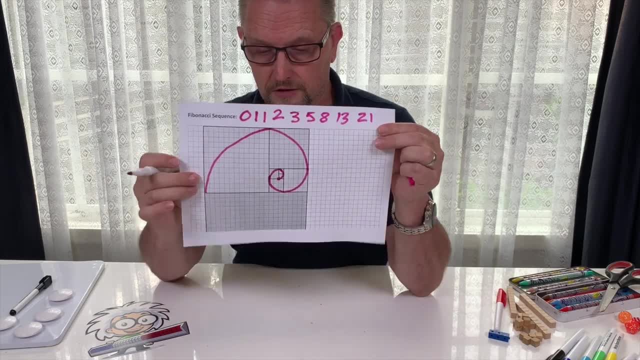 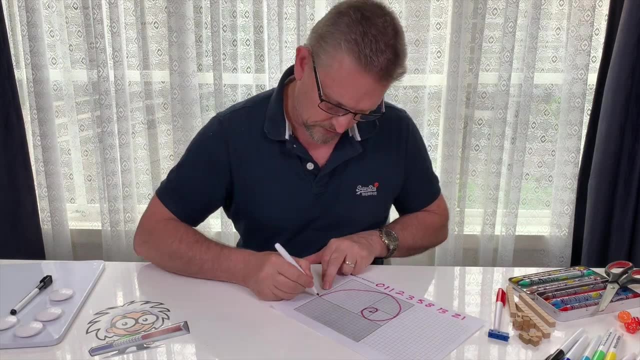 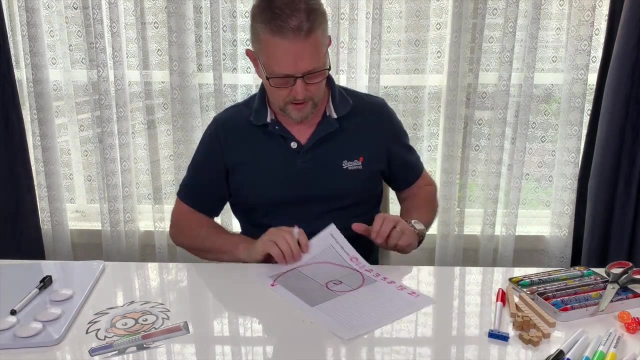 a larger piece of paper. you can do a fantastic spiral and you can see what's happening here. So I'm just going to follow that, curve around, Imagine where that you know that will be. So this will curve around here further like this and out over there. I'll put an arrow on that. 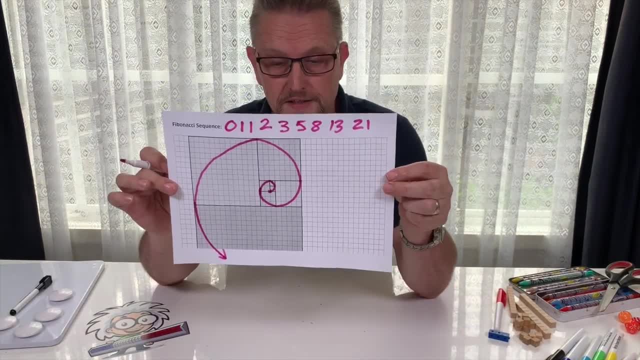 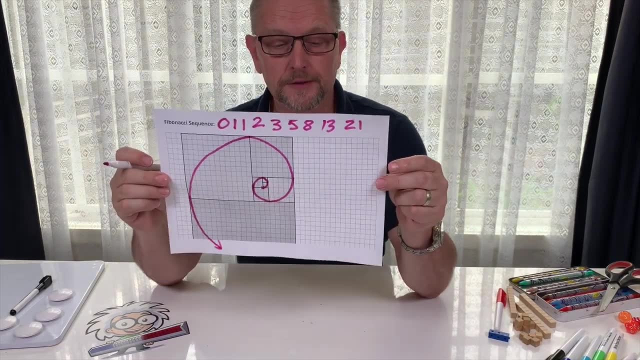 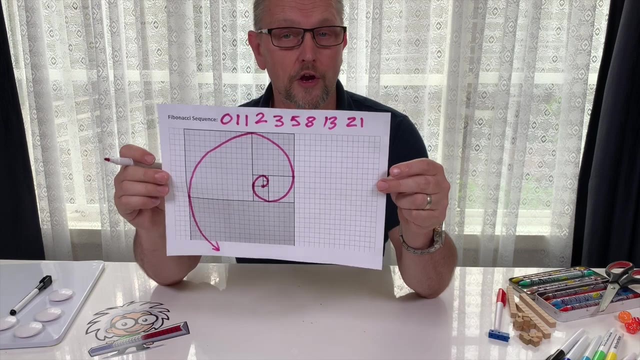 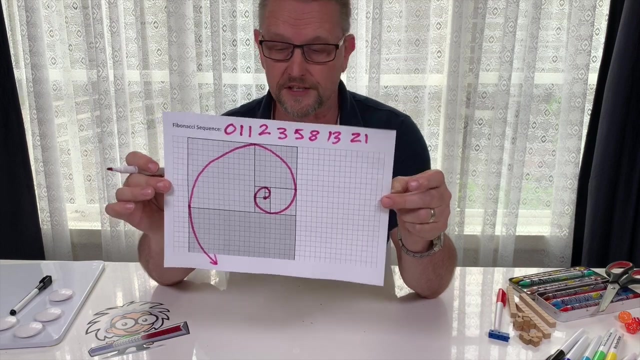 And you can see how how Fibonacci sequence is coming out when we put it on a bit of two-dimensional grid paper. It's amazing. And where would you find that? Well, I reckon you'd find that at no, in the ocean, say in a Nautilus shell. or down on the beach, say you know, seashells, sea snails. 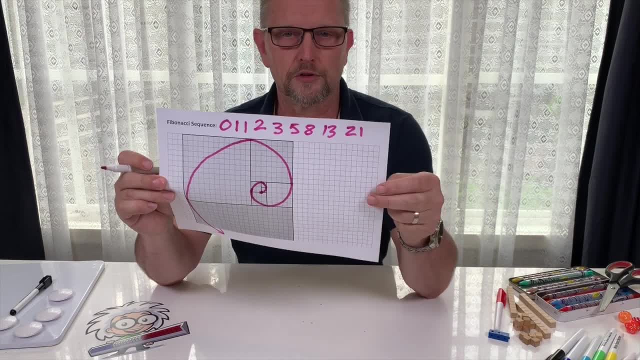 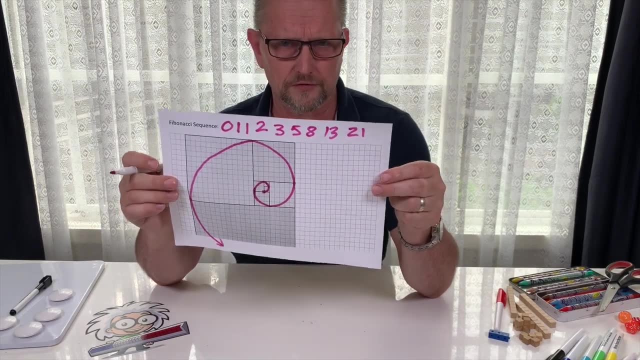 snails in the garden, All right. There's obviously things we use with different types of springs and stuff like that This sequence is used in, so with so many applications for the Fibonacci sequence, and a great thing for the kids to discover and to muck around with and try and understand that. 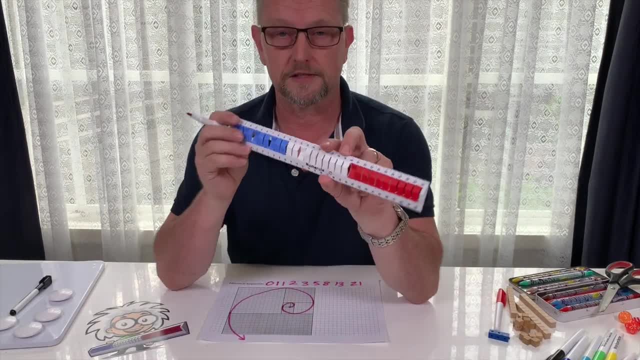 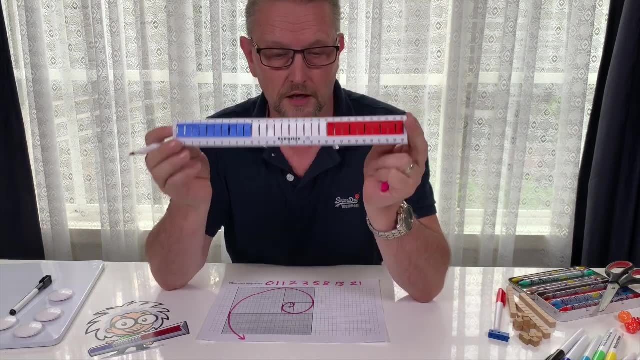 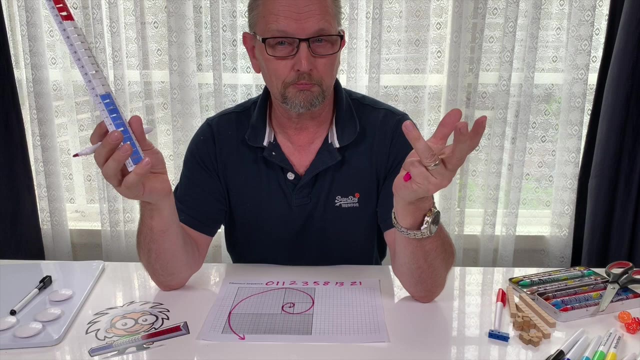 concept. So there it is. There's the Fibonacci sequence with the numeral. Now you can't tell me that that's not a complex thing that you can do with your kids and it's easy to manipulate and easy for them to understand. So Fibonacci sequence with the numeral. Okay, Hope you enjoyed. 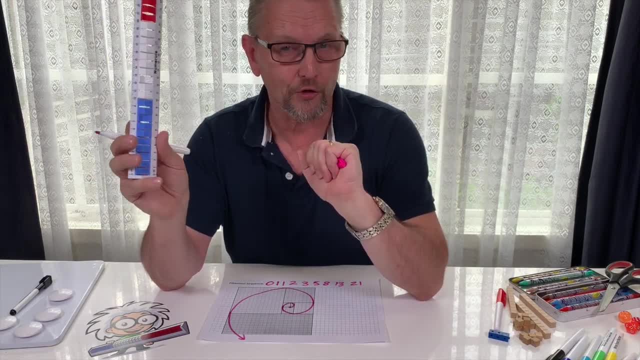 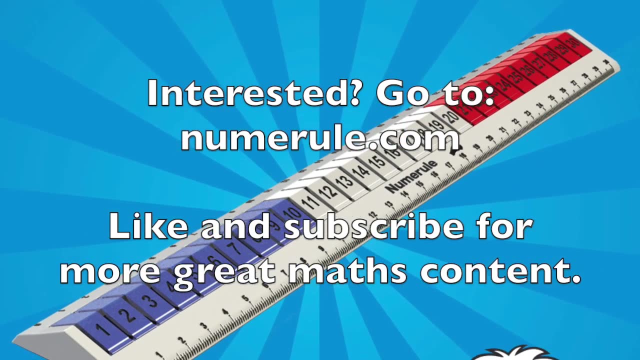 it. Have a great day and I'll see you next time. Thanks, See you, Bye.